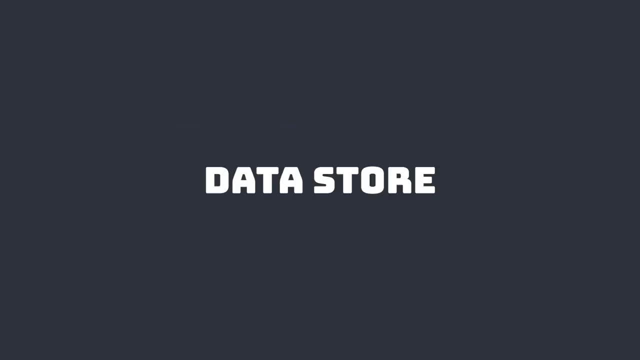 Vuex is one of the most popular ways in Vue to create a data store. And this means that our Vue app has one singular source of truth that's used in our Vue components. And when we want to change 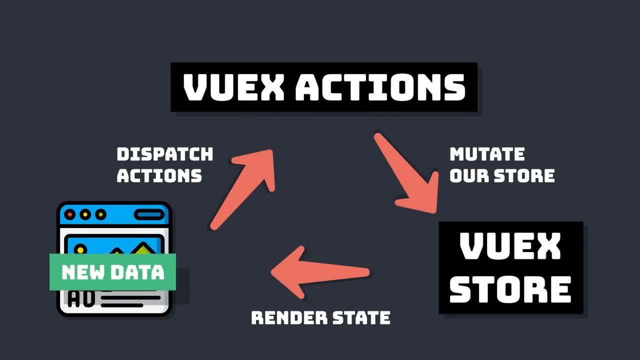 the state, we have a predictable one directional data flow to do this. Not only does this ensure that data across multiple components stays the same, but it also helps with dev tooling. So we 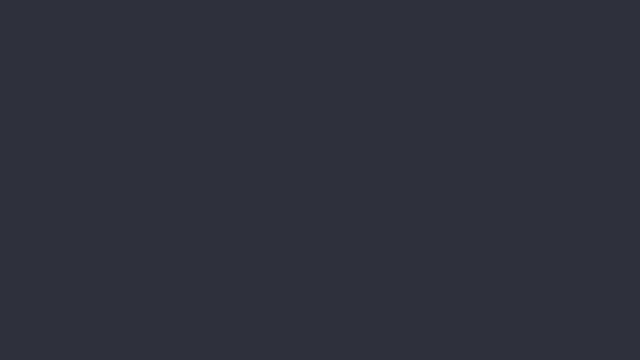 can see exactly how and when our data is being changed. For this video, I'll assume that you know a little bit about Vuex, but if you want a true beginner level video, let me know in the 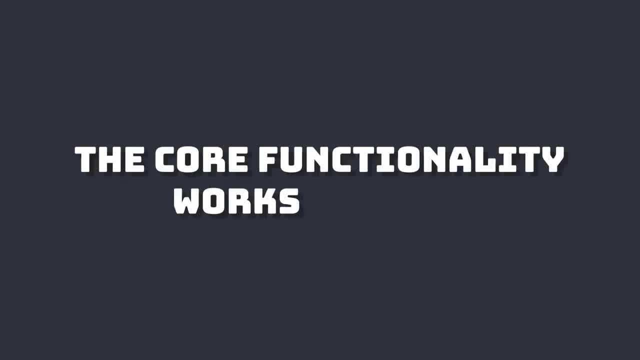 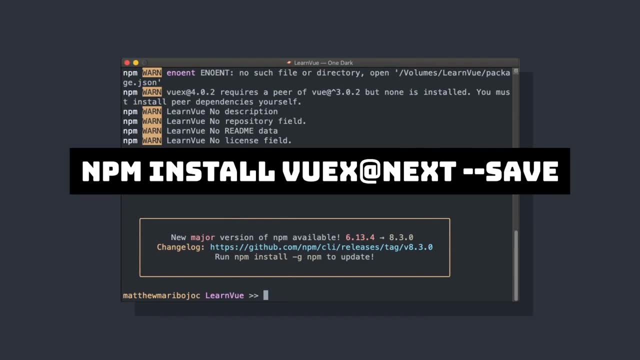 comments. But going back to Vuex, a lot of the core functionality is already great in Vue 3. To install Vuex into our Vue 3 projects, we can run npm install vuex-add-next-save. For example, 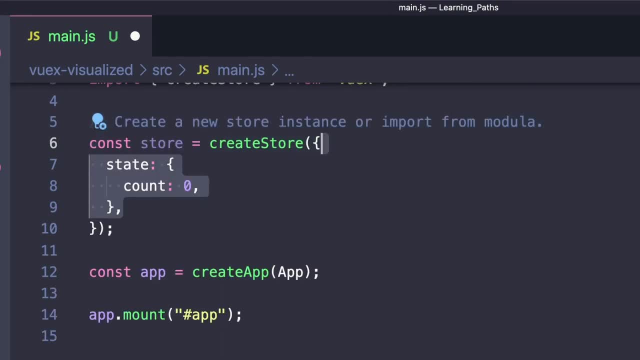 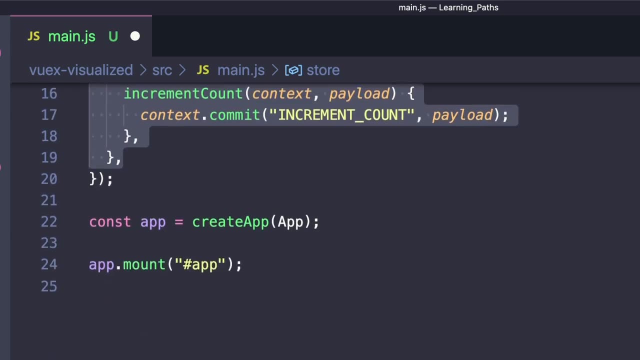 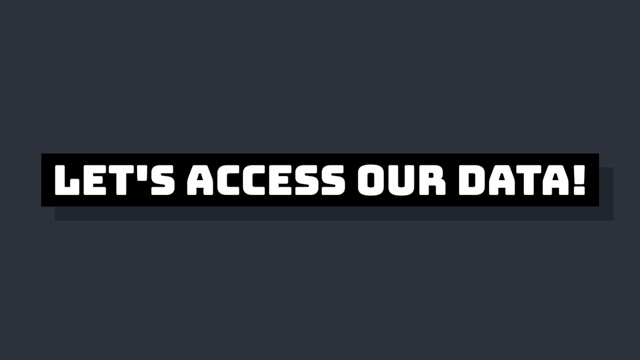 inside of main.js, we can add Vuex by creating a store and then adding our state, mutations, which are synchronous ways to change our state, and actions, which can be asynchronous and call mutations. And from here, we can tell our app to use our store. And that's all we need to do to get Vuex installed in our app. So let's create a component where we access our Vuex. And then we can add Vuex to our store. And that's all we need to do to get Vuex installed 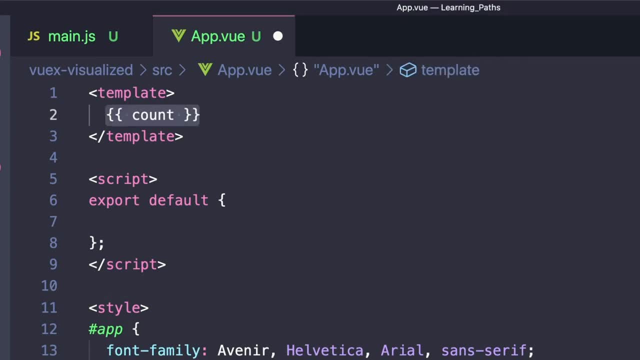 in our store. In our template, we'll include our count variable. And then inside of our script, we want to create a computed method. And it has to be computed to maintain reactivity. 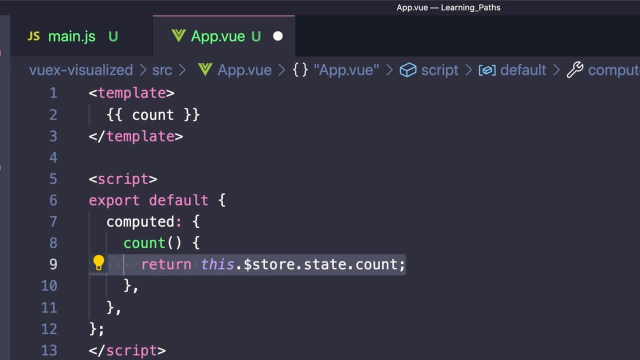 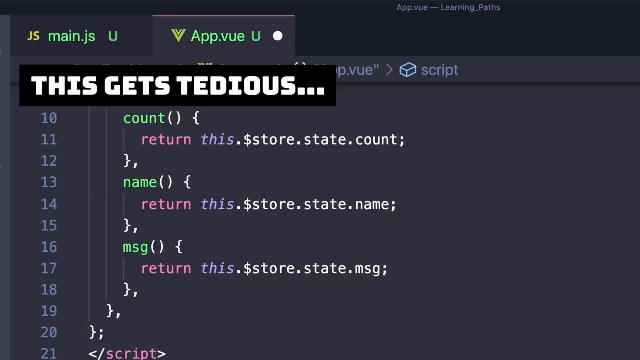 And inside of count, we'll return this.store.state.count. But let's say that we had other properties in our store, like a value for a name and a message. Instead of having to create individual properties for all of these, we can go back to our component and import map state from Vuex. And then we can set computed to map state and then pass in the property names from our store of the values we want in this component. 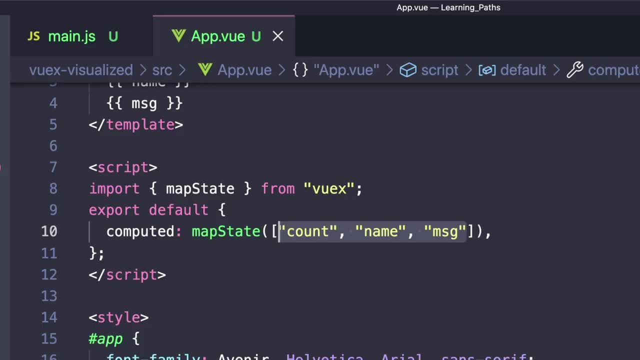 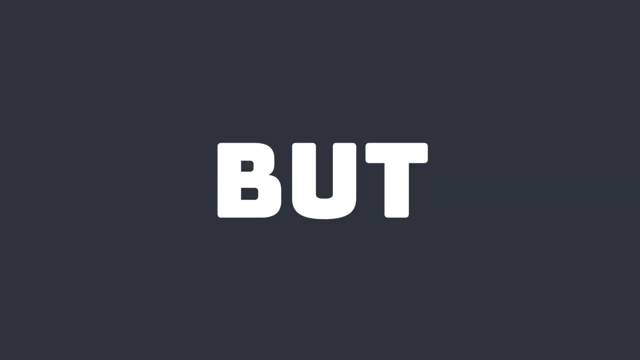 So for us, we'll say count, name, and message. This is a great concise way to access our store and also works for mapping actions, mutations, and getters. But if we switch over to the composition API, if we want to access a single property, we can do something similar. We'll 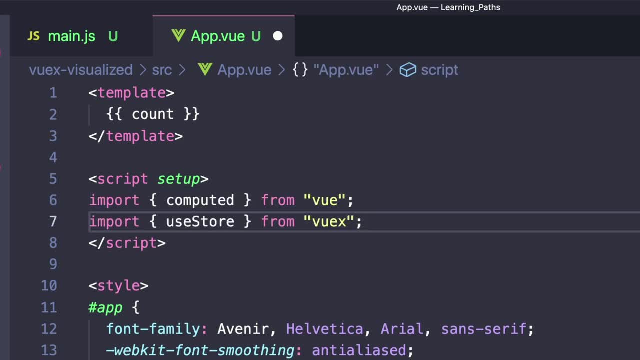 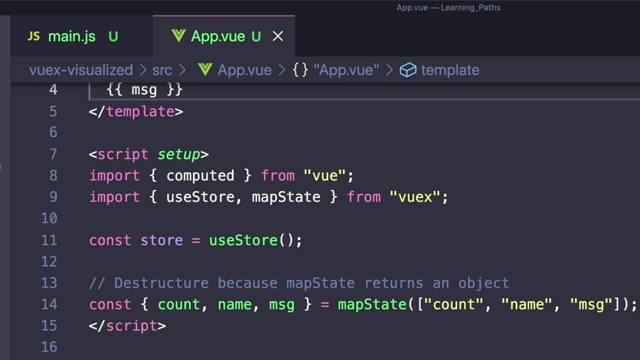 import computed from Vue and use store from Vuex. We'll create our store, and then we can create our computed property count. And inside, we'll return store.state.count. But let's see what happens if we use map state from Vuex. So we'll import it, and we'll say, const count, name, and message, and pass in our map state like we did with the options API.